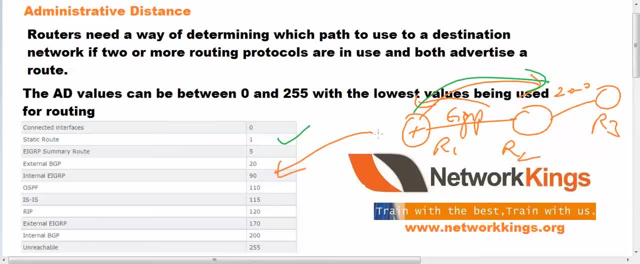 So static has one AD value. So static route will be shown in routing table as compared to EIGRP. EIGRP is 90 and AD value of static is 1. So static route would be preferred. So same for like OSPF is 110 and RIP is 120 and BGP is 20, 200.. So all as compared to static route they are: 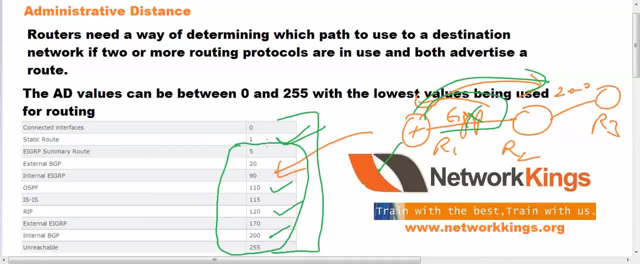 So higher AD value as compared to static route. So static route is preferred and for directly connected AD value is 0. So the AD values can be between 0 to 255 and routers need a way of determining which path to use to a destination network If two or more routing protocols, like I told you, from here I am getting a root of EIGRP and also have root of static, So both advertisers, same root. 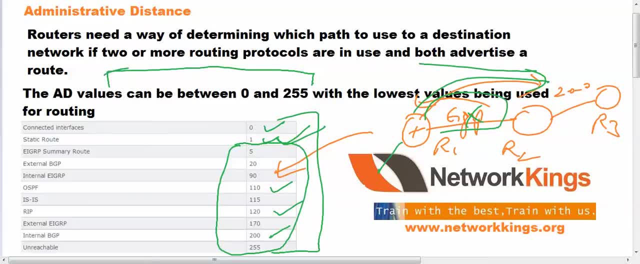 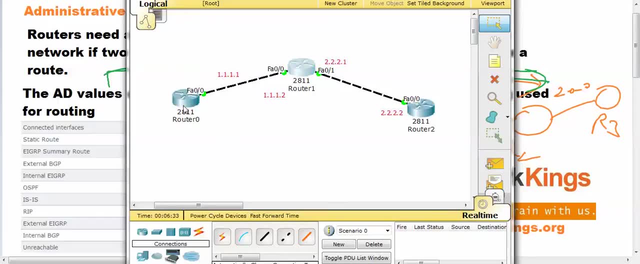 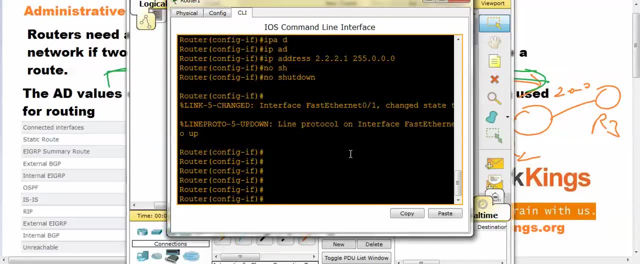 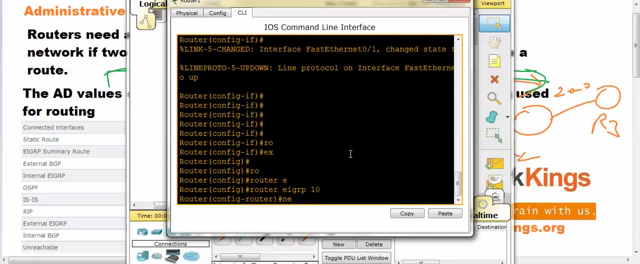 So in this scenario I have already configured IP addresses here, So let's configure EIGRP. So router EIGRP 10, network 1.0.. No auto summary. So in second router I am configuring router EIGRP 10, network 1.0.0.0, and this router also have 2.0.0.0. 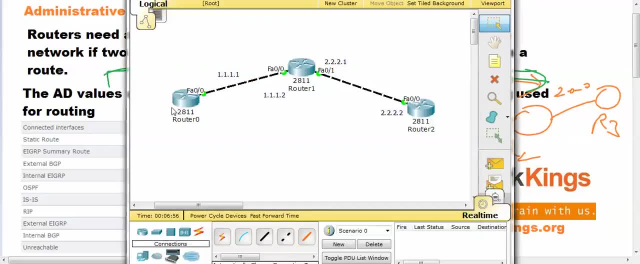 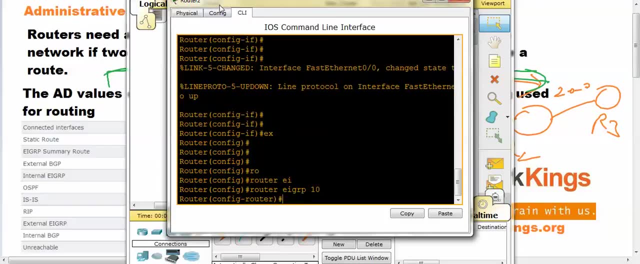 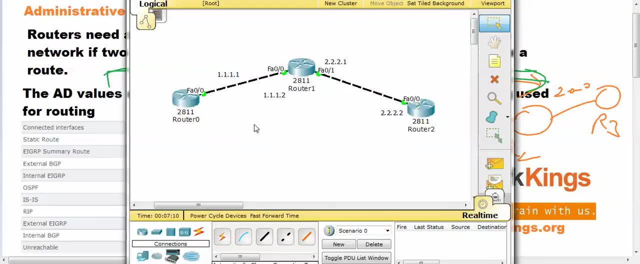 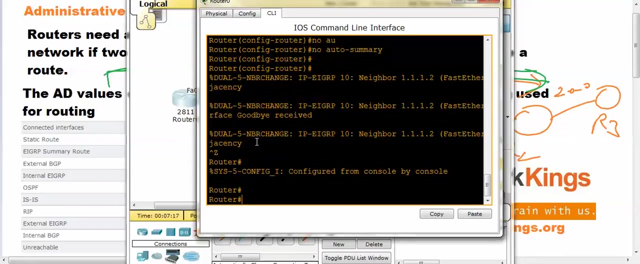 no autosummary. and on last router, router eigrp 10 network 2.0.0.0- no autosummary. so i configured router eigrp on all of the routers, so i am getting route of 2.0, let's. 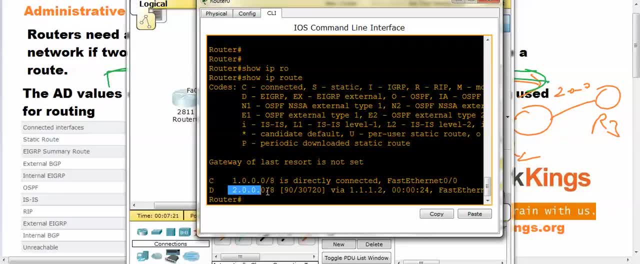 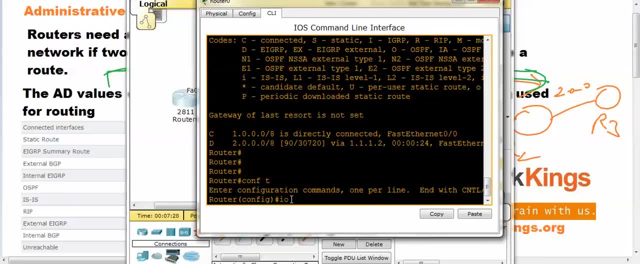 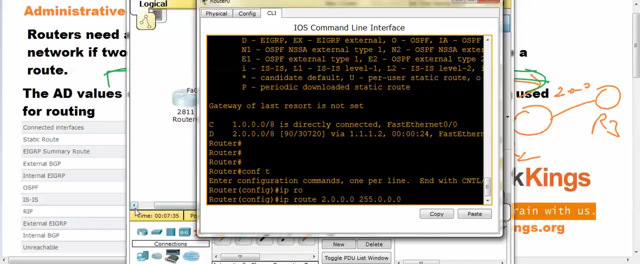 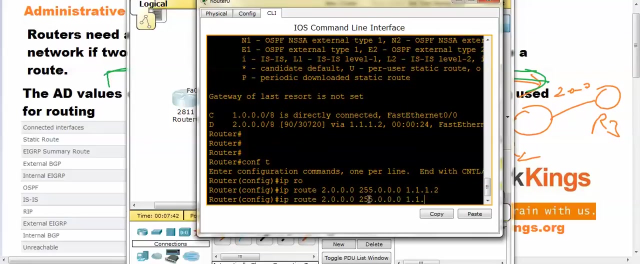 see. so i am getting 2.0.0.0.8 with ad value of 90. ok, and on this router, if i will set static route, ip route 2.0.0 with subnet mask and my neighbor is 1.1.1.2, you can also configure.